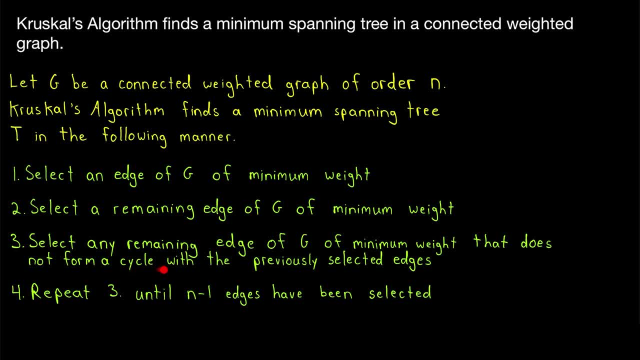 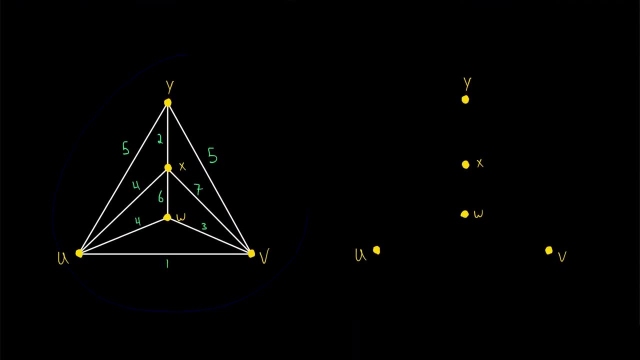 of minimum weight that does not form a cycle with the previously selected edges. Then we simply repeat step three until n minus 1 edges- The first one edges- have been selected and we get a minimum spanning tree. To make this algorithm more concrete, let's try running it on this graph here. This graph, as well as the next one we'll look at, are from a first course in graph theory by Chartrand and Zhang. I've pasted the algorithm here for our convenience. Remember that a spanning tree by definition contains all the vertices of the original graph, So the algorithm is going to select the edges. that will make the algorithm more concrete. 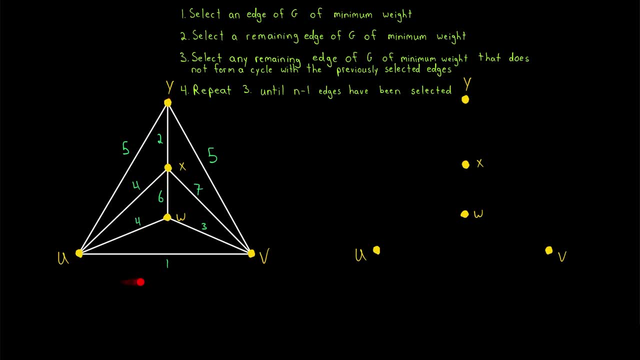 minimize the weight. So we'll run the algorithm on this graph, highlight the edges that we choose and then we'll actually draw those edges in over here, where I have duplicated the vertices of the graph, Note that the weight of each edge is written next to it in green. All right, step one is to select an edge of g of minimum weight. Looking through our edges, we see that the edge of minimum weight is this edge, with weight 1 joining u and v. So we'll go ahead and add that to the graph. 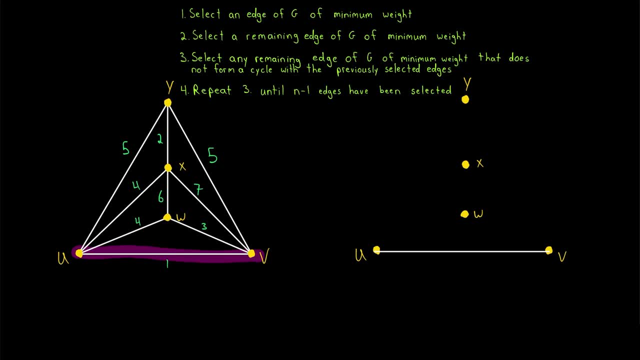 into our spanning tree, which we're keeping track of on the right. Step two: of the remaining edges, select one of minimum weight. Note: at this point we can select any edge of minimum weight, because it's impossible that we'll create a cycle with just two edges. Looking through the edges that remain, the edge of minimum weight is this one, with weight 2 joining y and x. Step three is just what we've been doing: Select a remaining edge of minimum weight. except now we have to only consider edges. 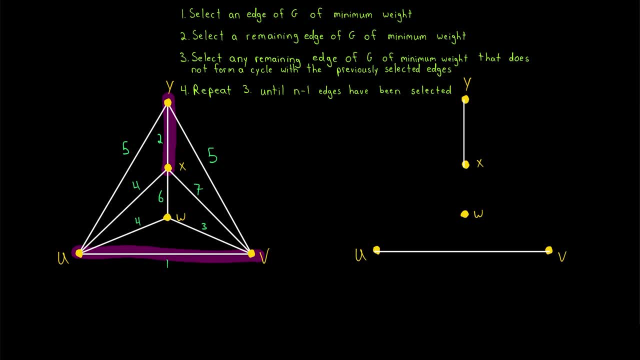 that will not produce a cycle with the edges we've already selected. Of the remaining edges, the edge of minimum weight is this, one of weight 3, joining w and v, And it does not create a cycle with our previous edges. So that is the next edge of our spanning tree And remember, we will repeat this step three until n minus one edges have been selected, One less edge than we have vertices, because it is at that point we will have completed our spanning tree. 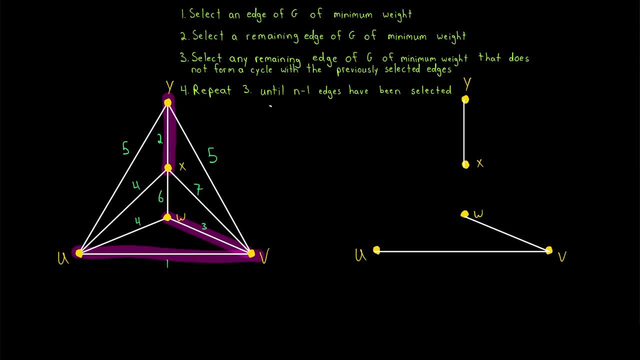 In, In this case, n. the number of vertices of the graph is 5, so we need to go until we have 5 minus 1, or 4 edges. We already have 3 edges, so we've just gotta select one more. 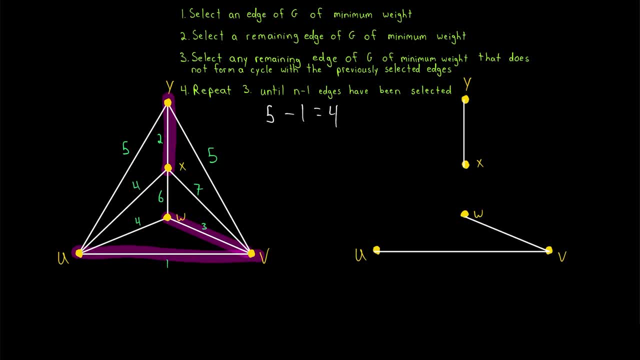 Again, of the remaining edges, we select one of minimum weight. that will not create a cycle. The edges of minimum weight are these two that both have weight 4,. however, we can't pick this one joining u and w, because that would create a cycle. 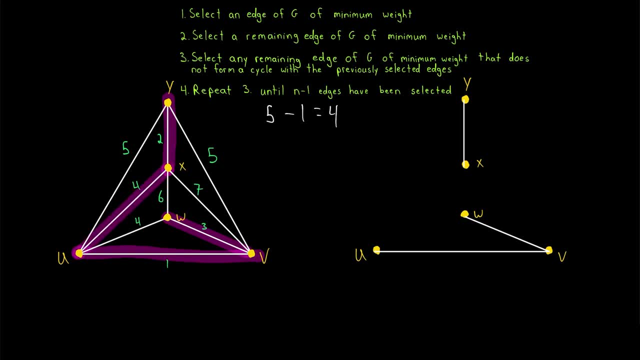 So the only edge we can choose is this one, joining u and x. Now that we have n minus 1, or 4 edges, we can stop and we have a minimum spanning tree. If we call this tree t, then w of t, the weight of the spanning tree, is equal to 10.. 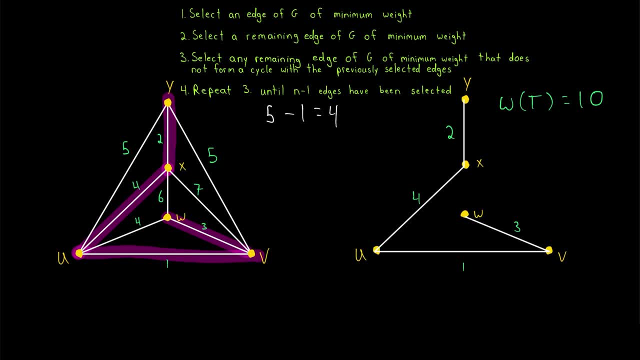 That's just the sum of the weights of the edges: 2 plus 4 plus 1 plus 3.. There are plenty of other spanning trees of this graph, but none of them will have a weight less than 10.. And that is the beauty of Kruskal's algorithm. 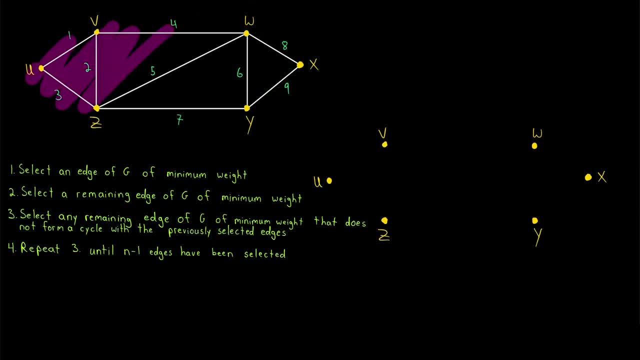 So that's how the algorithm works. try running it yourself on this graph to find a minimum spanning tree. Alright, did you do it? Did you find a minimum spanning tree? What's the weight of your tree? The weight of mine is 21, and of course, that should be the weight of yours, because there's 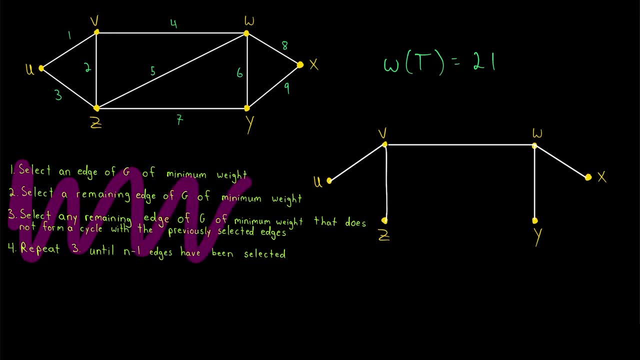 only one minimum weight. Remember that this algorithm can produce different minimum spanning trees from the same graph, since at times it is necessary to get the same number of edges to produce the same minimum spanning tree, to make an arbitrary choice among edges that are tied for the minimum weight. 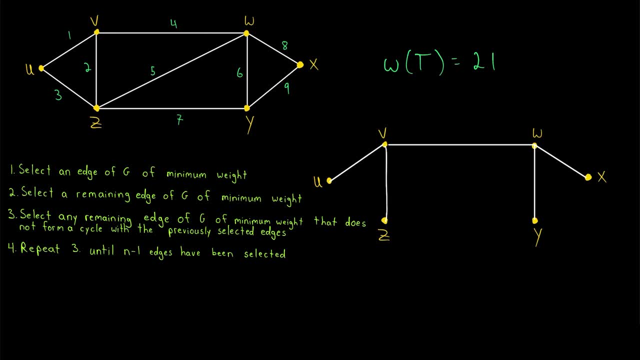 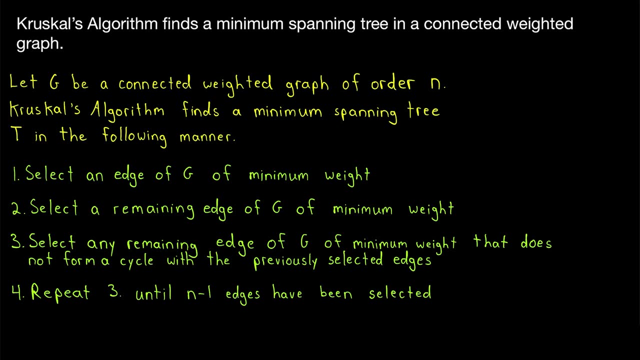 However, you won't encounter such a thing with this graph, so your minimum spanning tree should look like this. So that's Kruskal's algorithm for finding a minimum spanning tree. In a later video, we'll actually prove that the algorithm works. 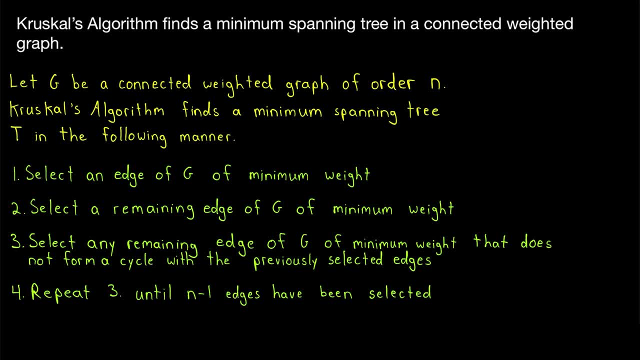 so we can be 100% sure it does what it's supposed to, And you can check the description for a link to that, as well as a link to my lesson on Prim's algorithm, which is a different, slightly more complicated algorithm for finding minimum spanning trees.